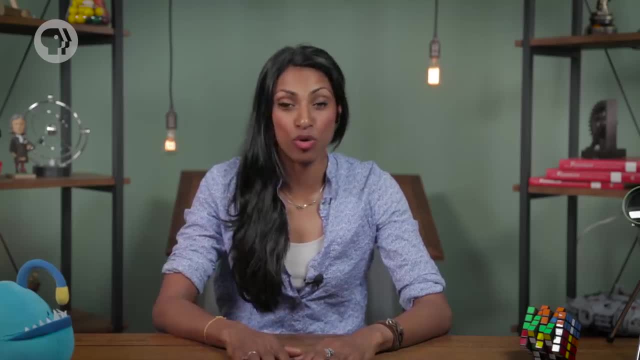 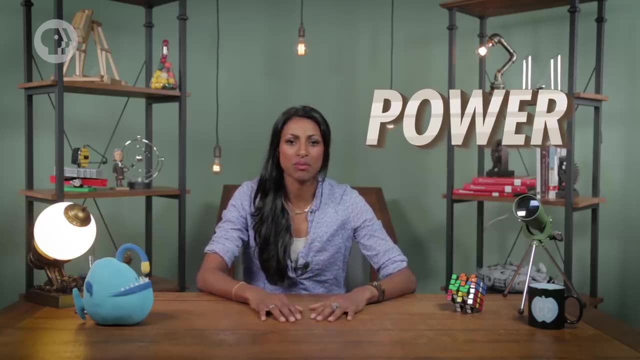 Today we're going to explore that definition and how it connects to one of the most important principles in physics – conservation of energy. We'll also learn what physicists mean when they talk about another concept that comes up a lot in daily life – power. So let's get to work. 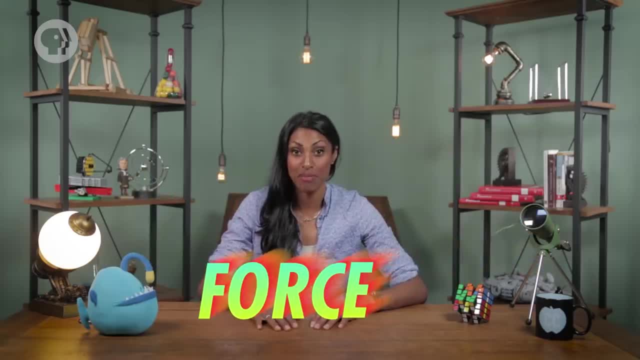 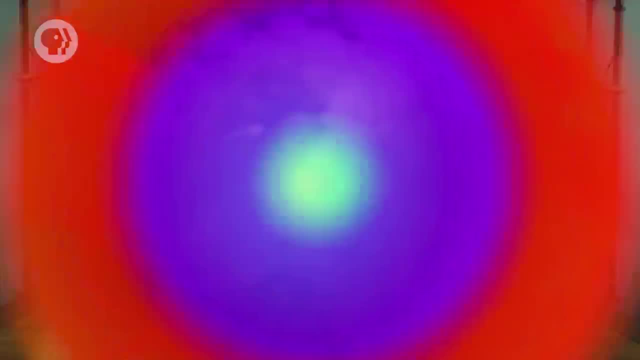 So far in this course, we've spent most of our time talking about forces and the way they make things move. You need to understand forces before you can understand work, Because work is what happens when you apply a force over a certain distance to a system. 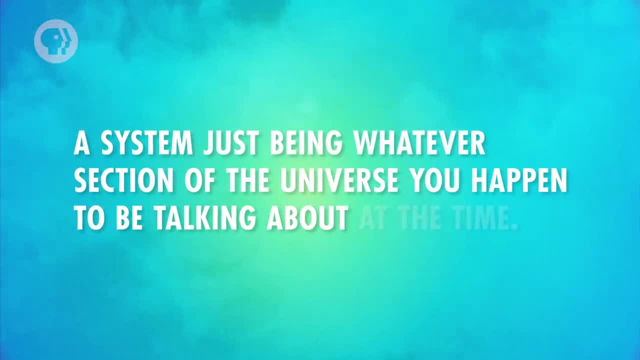 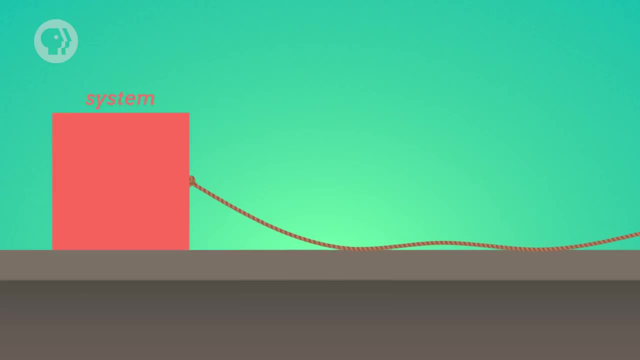 A system just being whatever section of the universe you happen to be talking about at the time. For example, if you're using a rope to drag a box across the floor, we might say that the box is your system and the force you're using to pull on it is an external force. 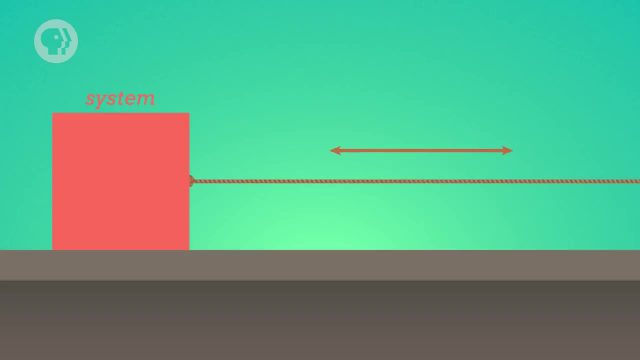 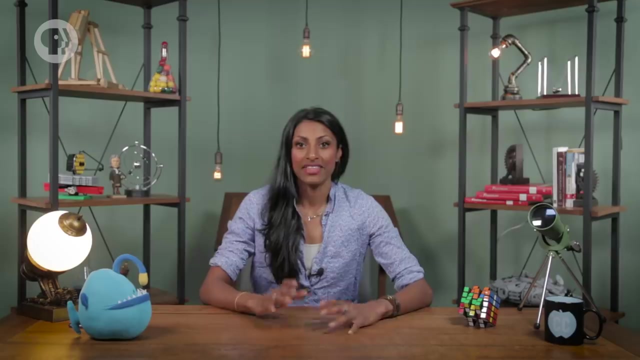 So let's say you're pulling on this box system by dragging it straight behind you, so the rope is parallel to the ground. If you're using the rope to pull the box for one meter, we'd say that you're doing work on the box. 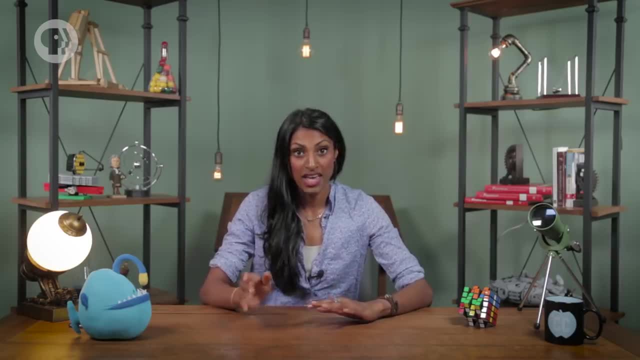 And the amount of work you're doing is equal to the force you're using to pull the box, times the distance you moved it. For example, if you pulled the rope, and therefore the box, with a force of 50 Newtons, while 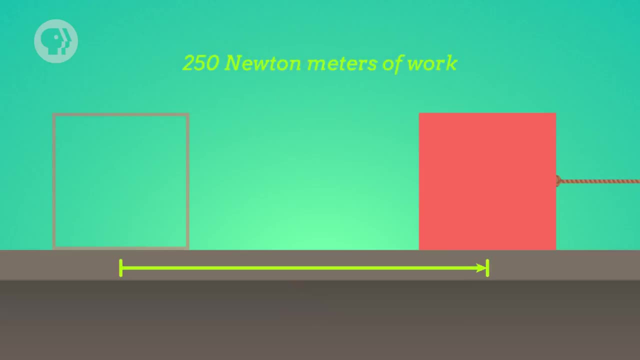 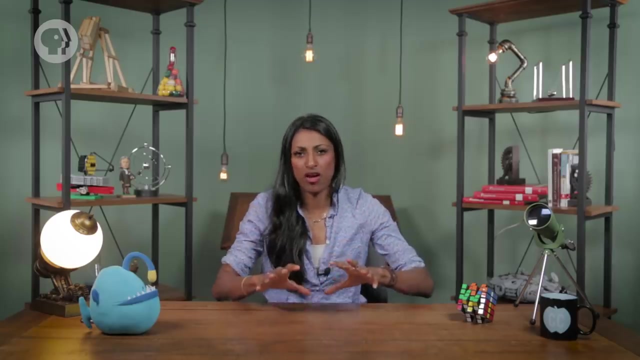 you moved it five meters, then we'd say that you did 250 Newton-meters of work on the box. More commonly, however, work is expressed in units known as joules. Now, sometimes the force you're applying to an object won't be in the exact same. 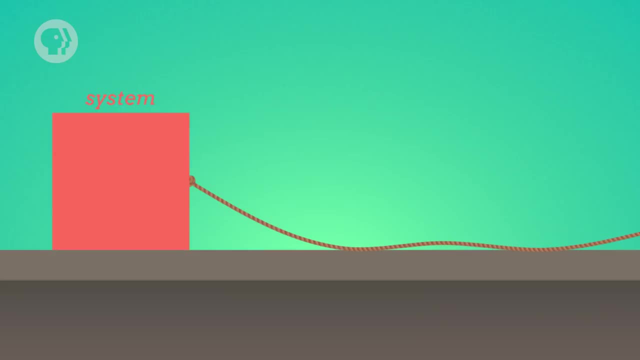 direction as the direction in which the object is moving, Like if you tried to drag the box with your hand higher than the box so that the rope was at an angle to the floor. In that case, the box would move parallel to the floor, but the force would be at an. 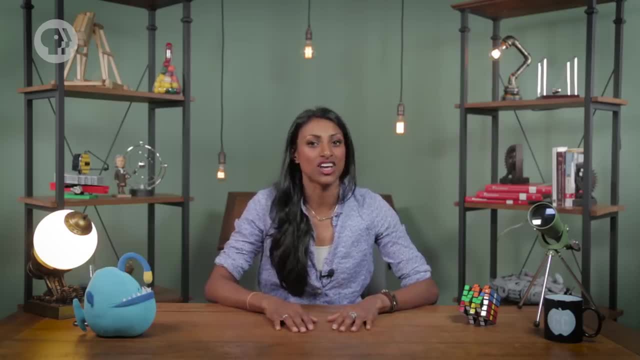 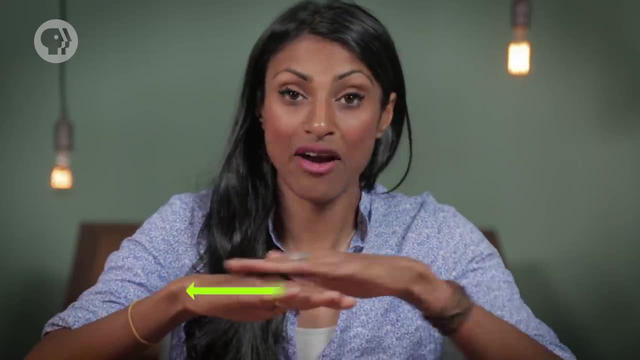 angle to it, And in such an instance you'd have to use one of the tricks we learned earlier, when we first talked about vectors. Specifically, you need to separate the force you're using on the rope into its component parts – one that's parallel to the floor and one that's perpendicular to it. 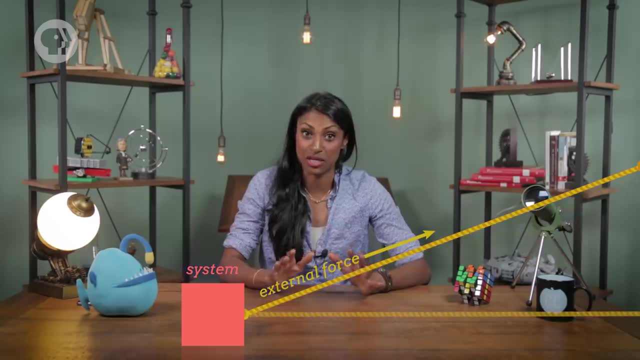 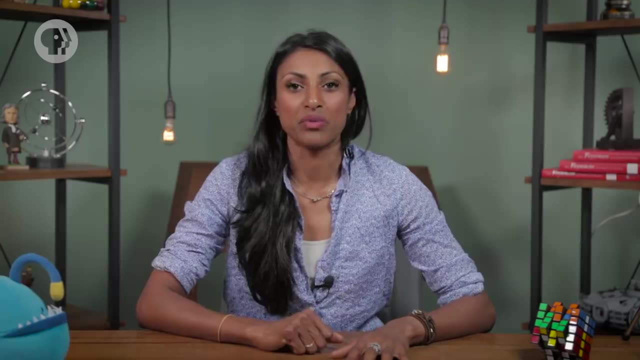 To find the part of the force that's parallel to the floor, that is the one that's actually pulling the box forward. you just have to multiply the magnitude of the force by the cosine of the rope's angle to the ground. You'll remember that we typically designate an angle in a system as theta. 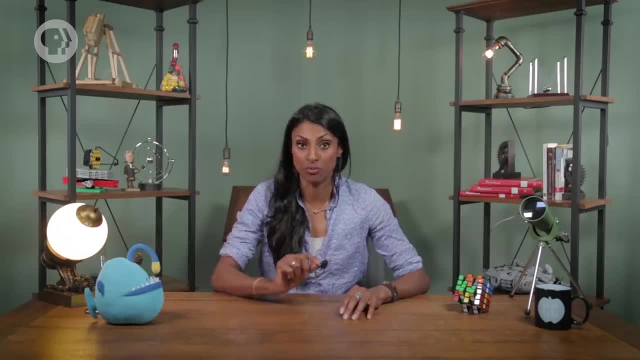 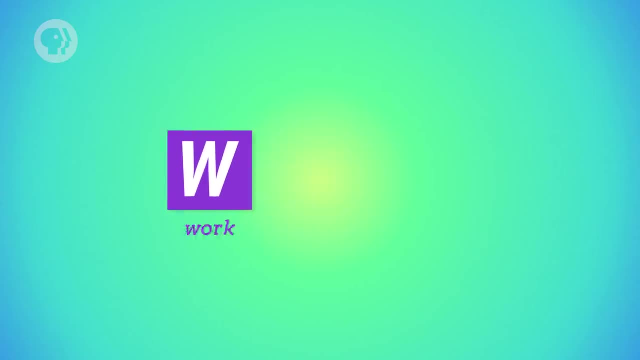 So to calculate the work you did on the box, you just multiply the horizontal component, or f times the cosine of theta, by the distance you moved the box. That's one way physicists often write the equation of work – they'll set it equal. 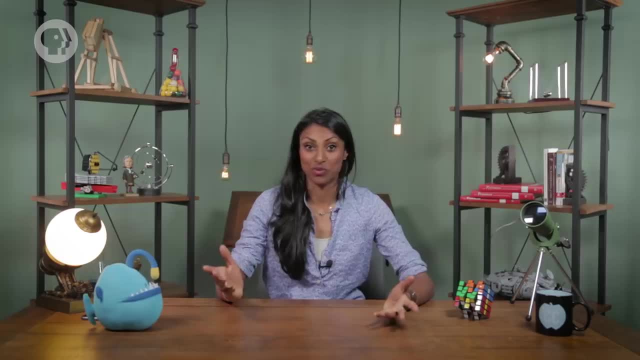 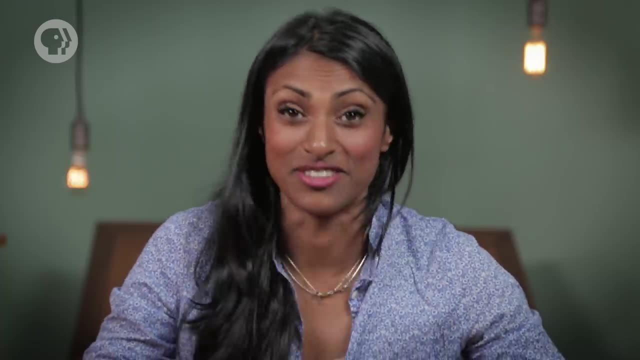 to force times, distance times, the cosine of theta, And that equation will fit any scenario that involves a constant force being applied over a certain distance. But what if that force isn't constant? What if, say, you started out pulling hard on the box, but then you started to get tired? 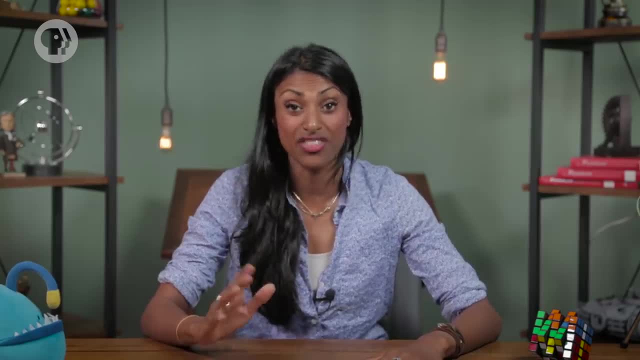 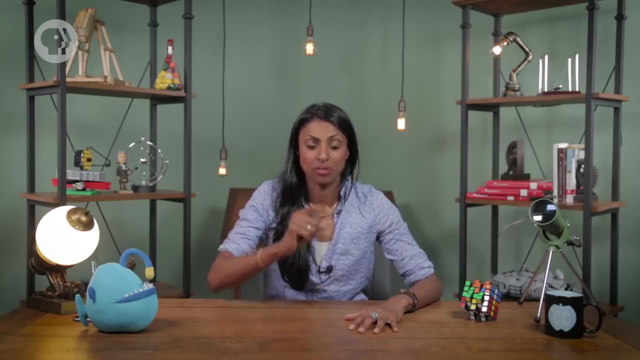 so the amount of force you exerted on the box got smaller and smaller the further you dragged it. To calculate the work you did in that case, you'd have to count up the amount of force you applied over each tiny little bit of distance. 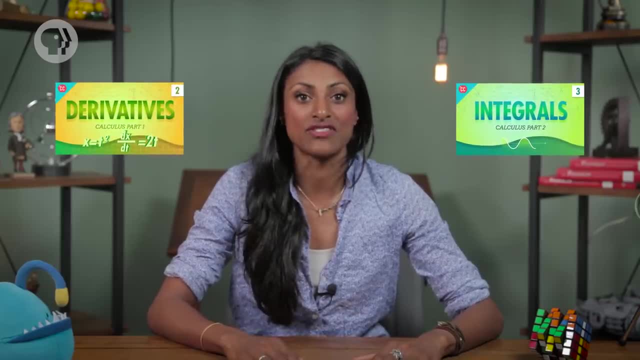 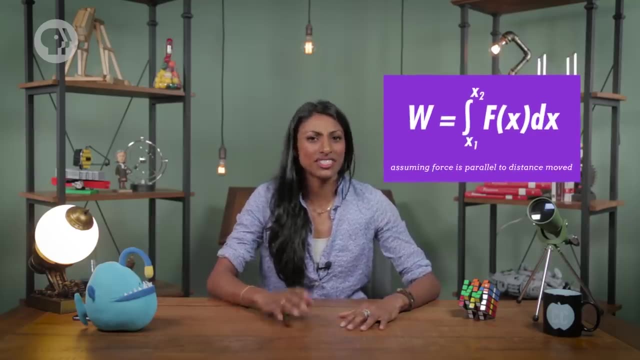 And if you've watched our episodes on calculus, then you'll know that there's a faster way to add together infinitely tiny increments – integration. So to find the work done by a varying force, you just have to integrate that force relative to the distance, the object moved. 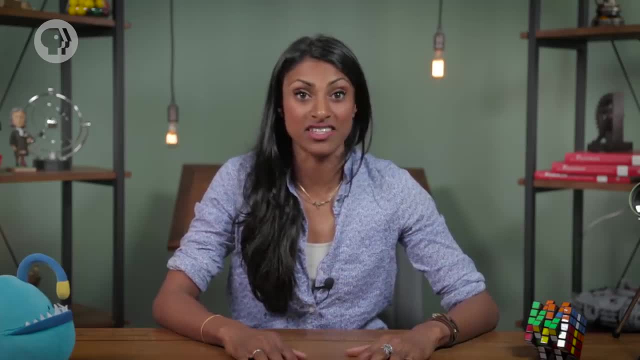 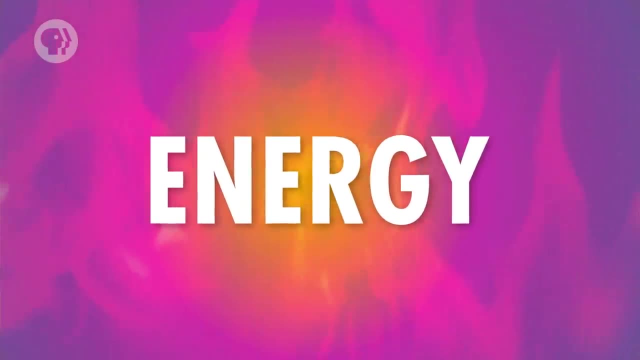 Which would look like this. But force times distance is only one of the ways that physicists measure work, Because you know how we just said that joules are the units of work. Well, joules are often used as the units for something else – energy. 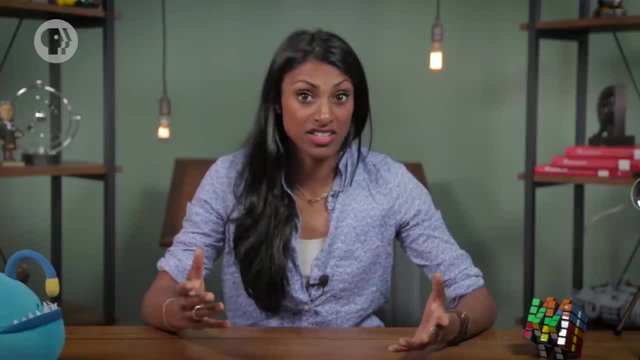 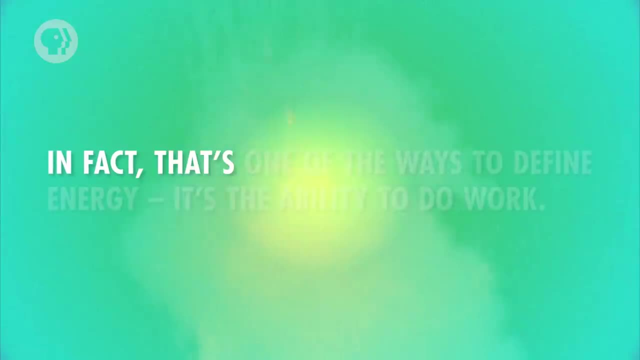 And work uses the same units for energy. It's what happens when an external force is applied to a system and changes the energy of that system. In fact, that's one of the ways to define energy – it's the ability to do work. 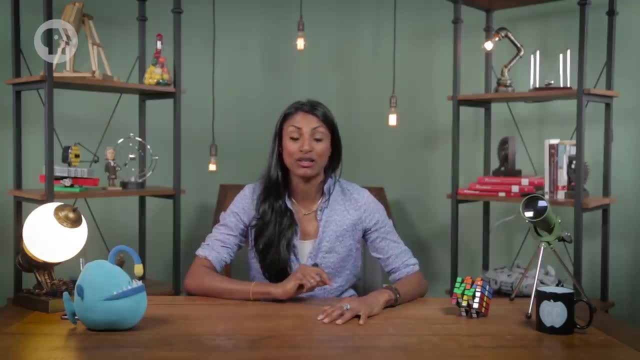 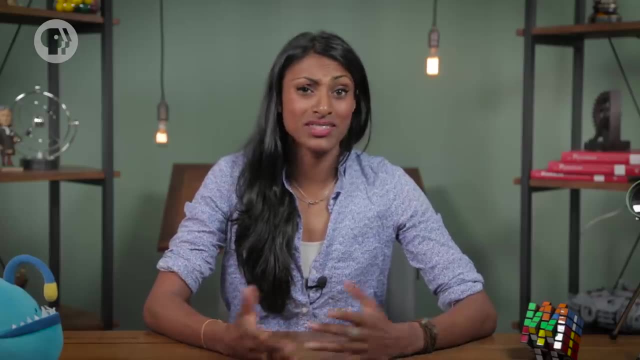 There are all different kinds of energy, but in this episode we'll mainly be talking about two of them – kinetic energy and potential energy. Kinetic energy is the energy of motion. When the box was resting on the ground, we'd say that it had no kinetic energy. 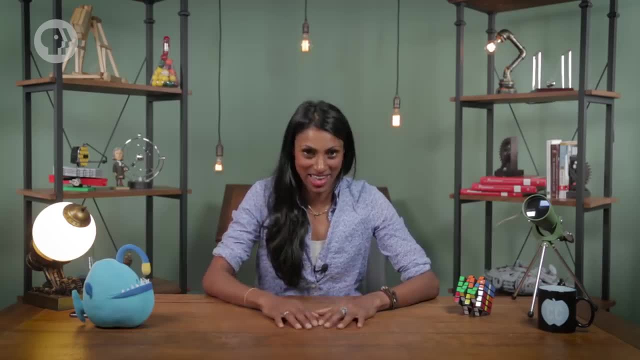 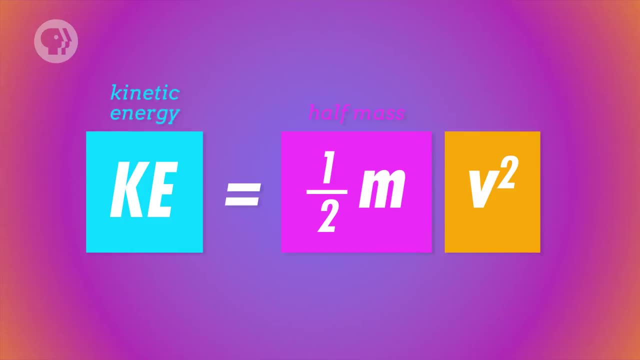 But once you applied a force and it started moving, it did have kinetic energy And the energy of the box changed, which means that you did work on it. More specifically, the kinetic energy of an object is equal to half of its mass times. 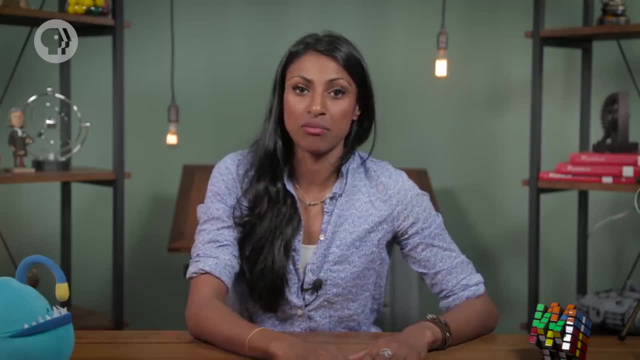 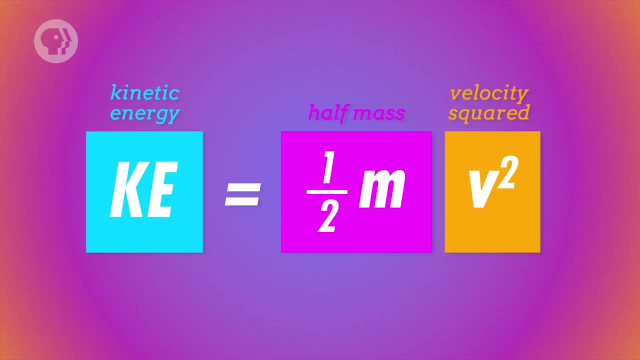 its velocity squared. If this looks familiar, that's because it comes from applying both Newton's second law and the kinematic equations to the idea that work is equal to force times distance. So if the box has a mass of 20 kilograms and at some point while you're dragging, 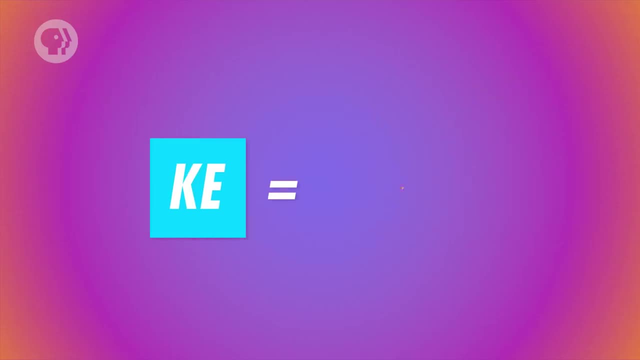 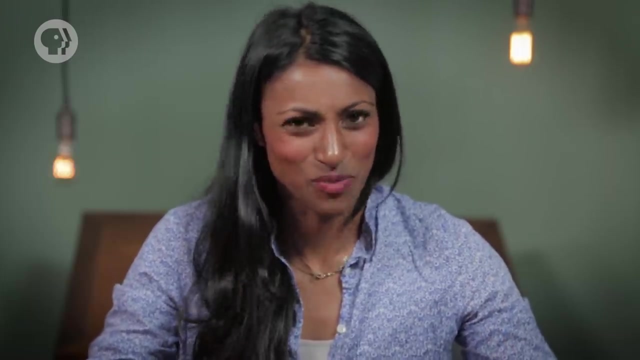 it, it reached a velocity of 4 meters per second. we'd say that its kinetic energy at that moment was 160 joules. Then there's potential energy, which actually isn't what it sounds like. Potential energy isn't potentially energy, it's potentially work. 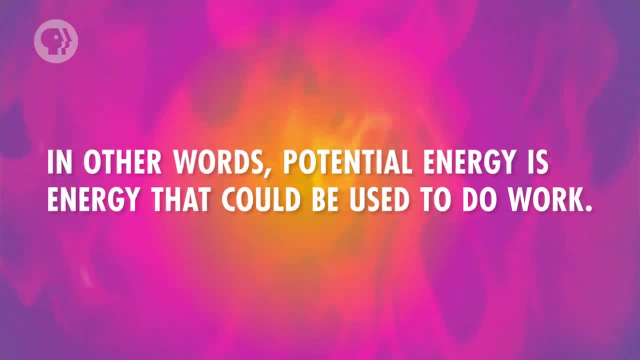 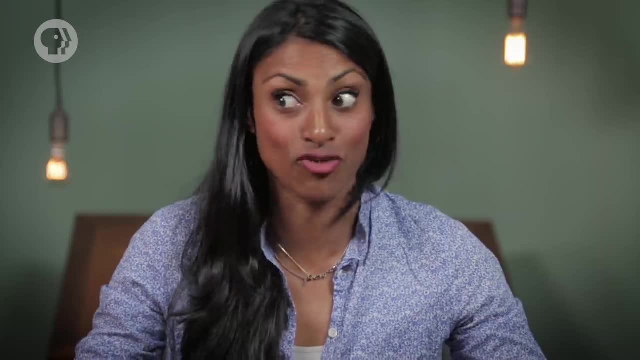 In other words, potential energy is energy that could be used to do work. One common type of potential energy is gravitational potential energy, Basically, the potential energy that comes from the fact that gravity exists. If I hold this book about a meter above the ground, we'd say that it's got gravitational. 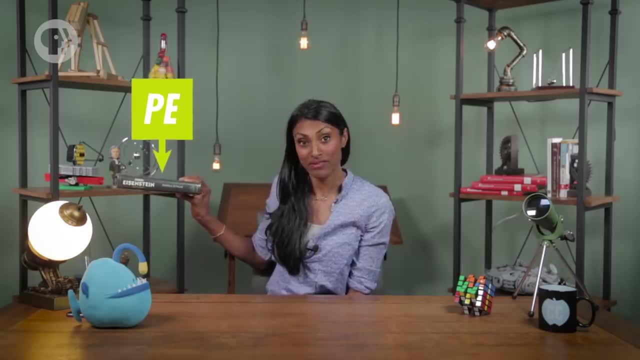 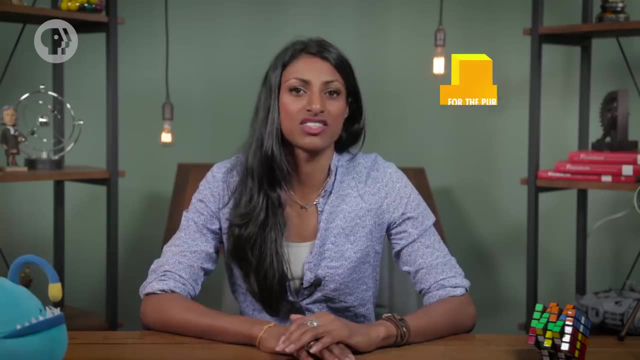 potential energy, Because, if I let it go, gravity is going to do work on the book. Gravity exerted a force that moved it to the ground. Once the book hits the ground, though, we'd say that its gravitational potential energy is zero, because gravity can't do work on it anymore. 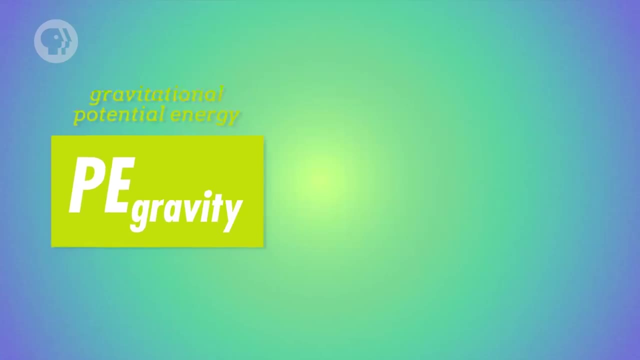 Calculating gravitational potential energy is easy enough. It's just the force of gravity on the object. so the object's mass times, small g, multiplied by the object's height, or mgh for short. Which means that just by knowing that this book's mass is about a kilogram and that 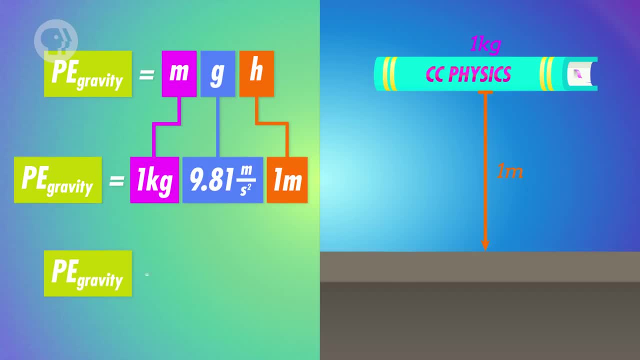 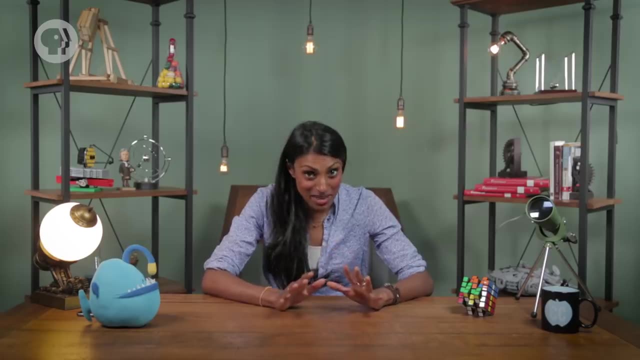 we held it about a meter above the ground. we can calculate the force of gravity on the object. We can calculate its potential energy, which is 9.8 Joules. Another type of potential energy that shows up is spring potential energy. Despite its name, it's not a seasonal thing. And yes, I really made that joke. Rather, it's the type of potential energy that's specific to springs. The force of a spring is equal to the distance by which it's either compressed or stretched times a constant that we write as k. 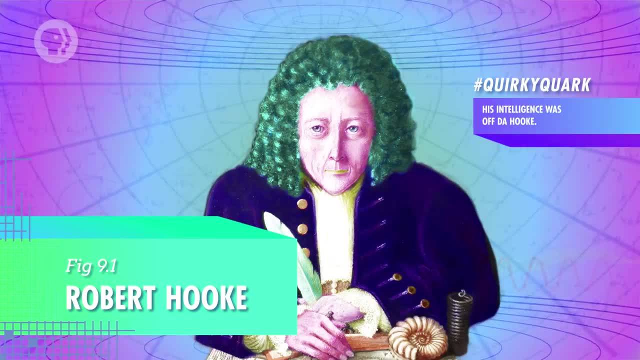 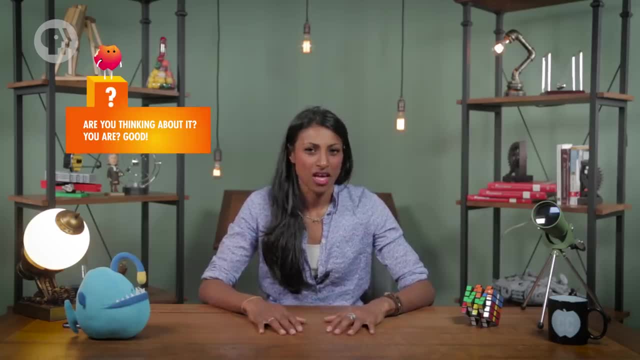 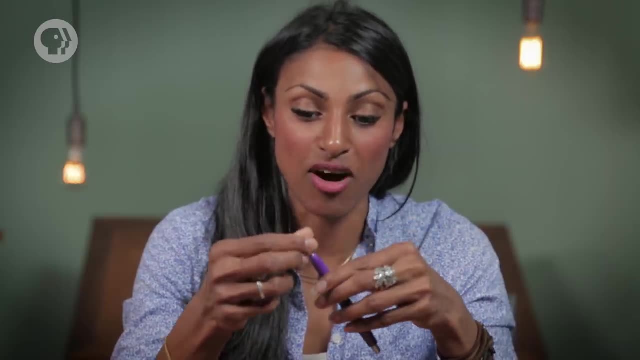 The equation makes sense if you think about it. The further you push on a spring and the stiffer it is, the harder it will resist. You can even test this out for yourself by taking apart a clicky pen and playing with the spring inside. 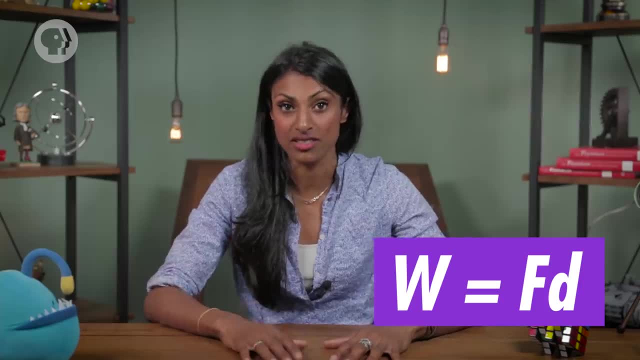 You can even test this out for yourself by taking apart a clicky pen and playing with the spring inside. By combining Hooke's Law with the idea that work equals force times distance, we can find the potential energy from a spring. It's half times k times the distance squared. 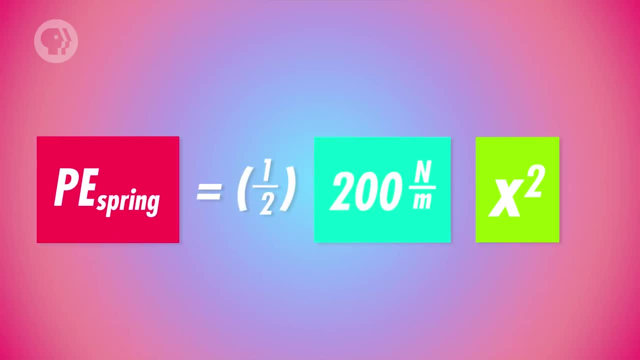 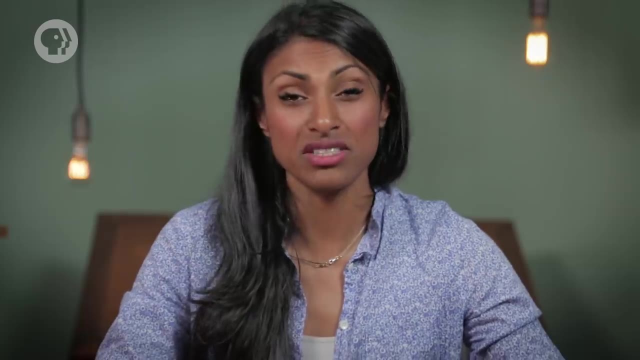 For example, if you have a spring with a spring constant of 200 Nm and a block is compressing it by half a meter, then the potential energy of the block would be 25 Joules. So when something does work on a system, its energy changes. 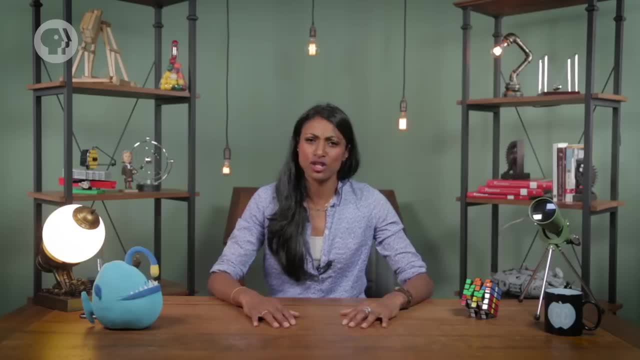 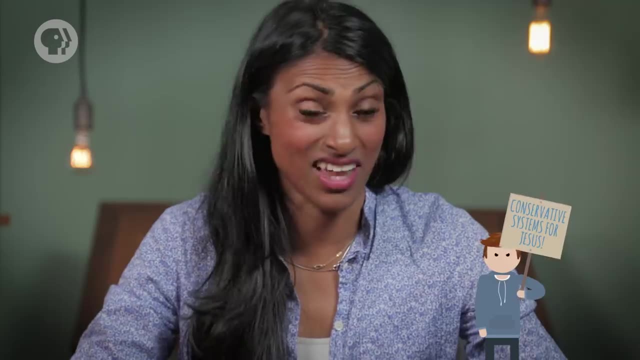 But how that energy changes depends on the system. Some systems can lose energy, and these are known as non-conservative systems. Now, that doesn't mean that the energy that's lost is literally disappearing from the universe, And it doesn't have anything to do with the system's personal politics either. 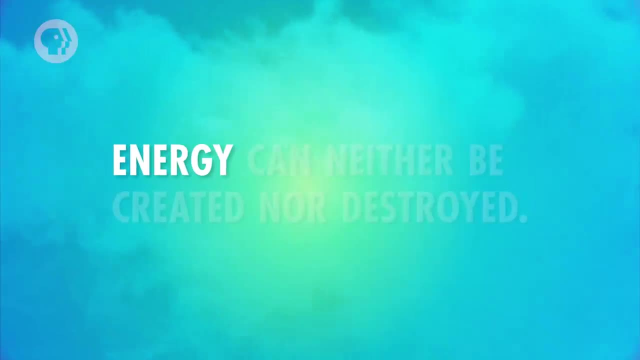 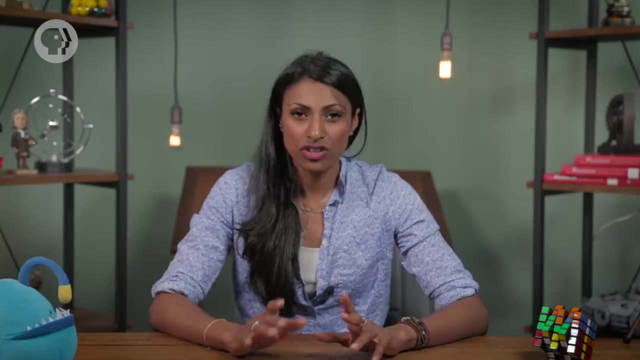 It just relates to one of the most fundamental principles of science: that energy can neither be created nor destroyed, But systems can lose energy, Like when friction from the box breaks. Dragging on the floor generates heat To non-conservative systems. you can still talk about their kinetic energy or potential. 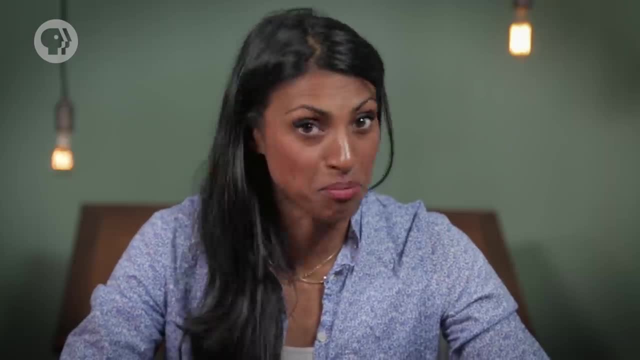 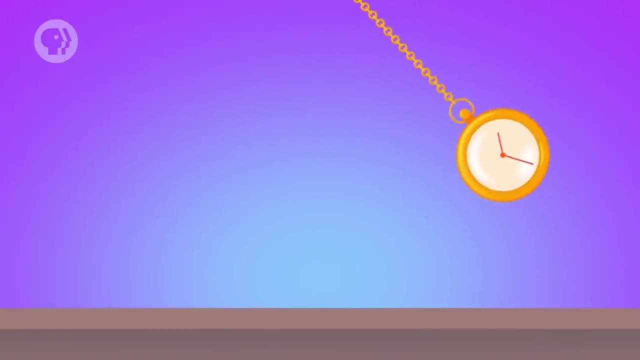 energy at any given moment. But conservative systems, let you do much more than that. A conservative system is one that doesn't lose energy through work. Say a simple pendulum: When the pendulum is at the top of its swing, it stops moving for a brief moment as it changes. 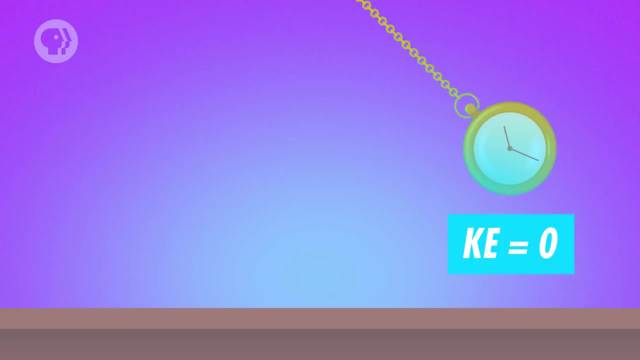 direction, meaning that its kinetic energy at that point is zero. But it has lots of potential energy because the gravitational force can do work on the pendulum. It can pull the pendulum down until it reaches the bottom of its swing. At the bottom of the swing that potential energy becomes zero, because gravity can't. 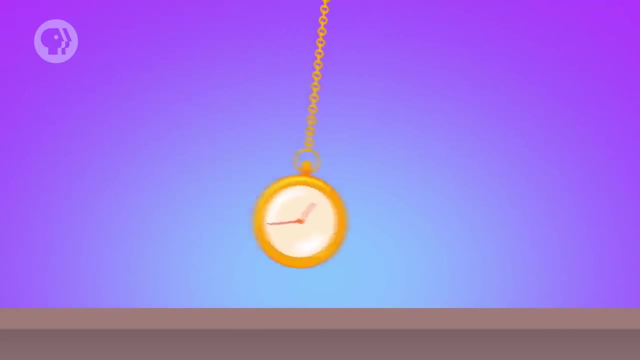 pull the pendulum down anymore. But now the pendulum has lots of kinetic energy because it's moving through the swing And it turns out that at any given point in the pendulum's motion its kinetic energy and potential energy will add up to the same number. 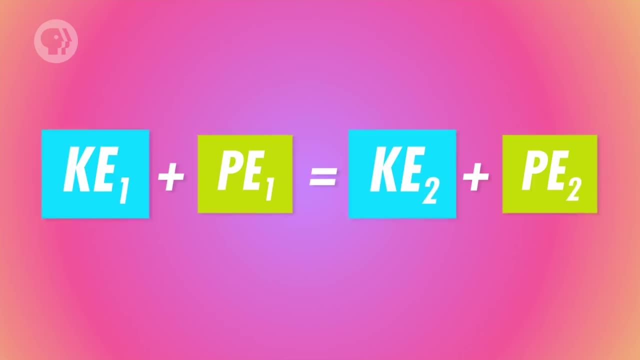 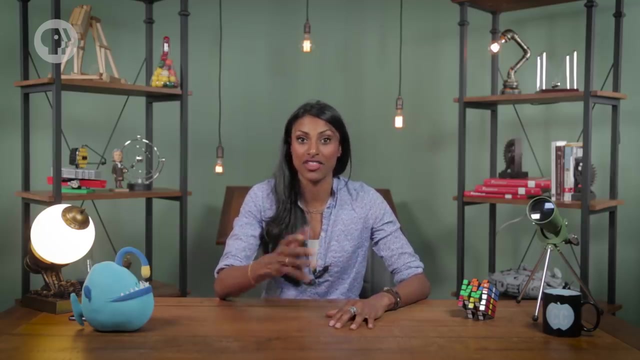 If its potential energy increases, its kinetic energy will decrease by the exact same amount, and vice versa. So now that we know how to define work, we can use that definition to help explain another common term that physicists have a very specific meaning for – power. 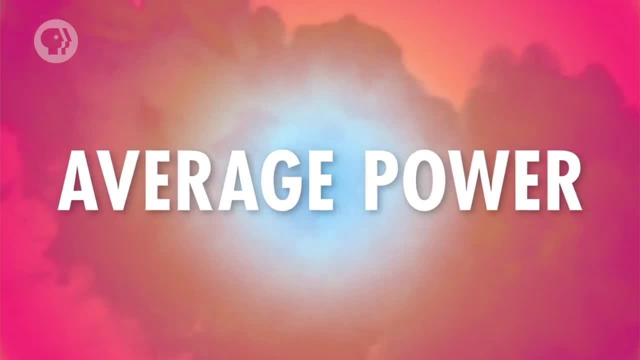 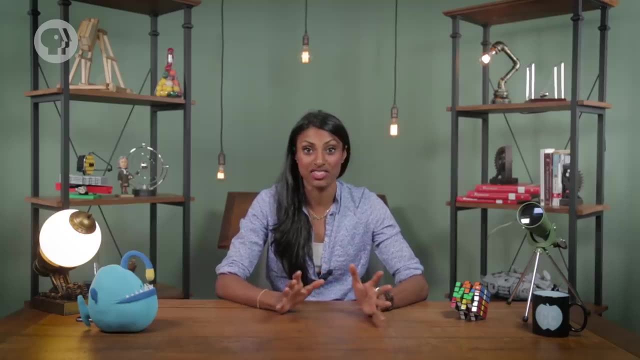 Or, more specifically, average power. Average power is defined as work over time and it's measured in watts, which is just another way of saying joules per second. Basically, it's used to measure how much energy is converted from one type to another. 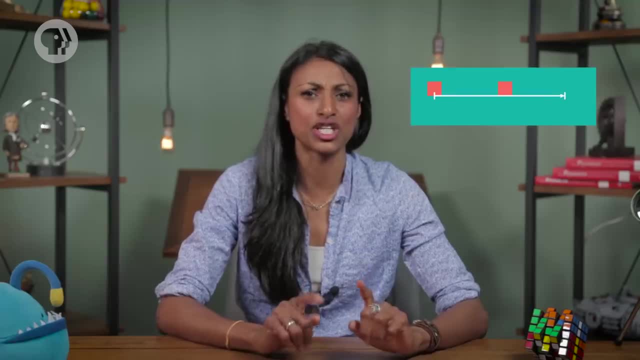 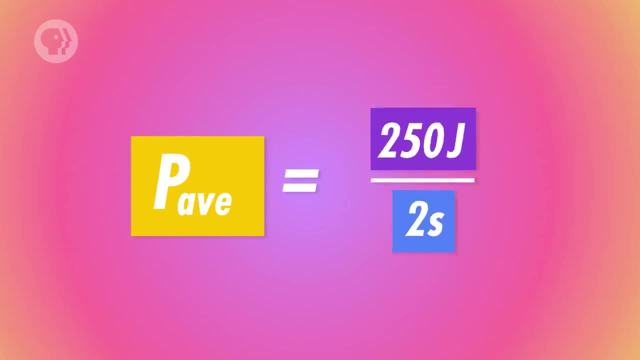 over time. So remember that box you were pulling. We figured out that you did 250 joules of work on the box when you moved it 5 meters. If you took 2 seconds to move the box, then your average power output was 125 watts. 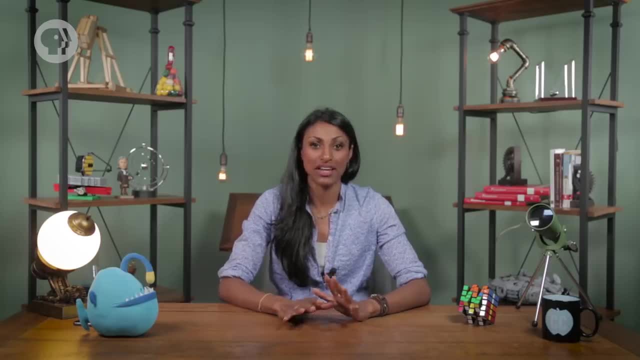 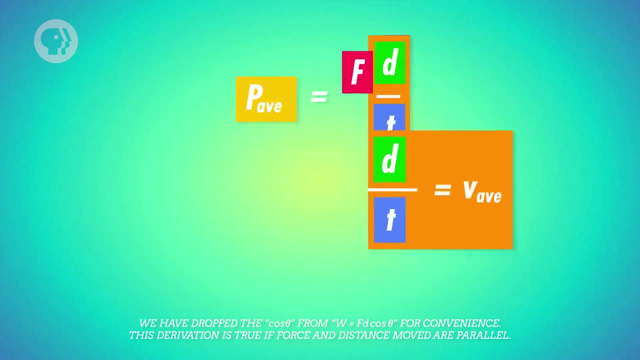 You're basically doing the same thing. You're basically a light bulb. Now we can also describe power in another way by putting two different facts together: that work is equal to force times distance, and that average velocity is equal to distance over time.